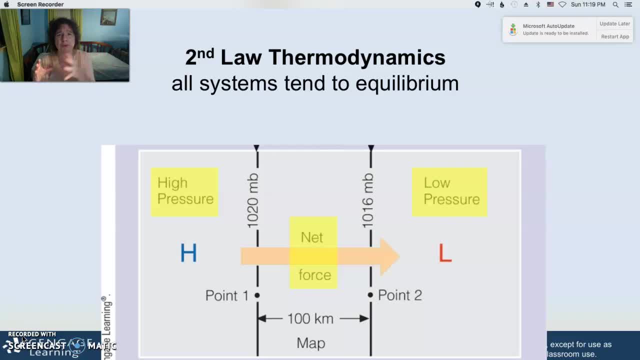 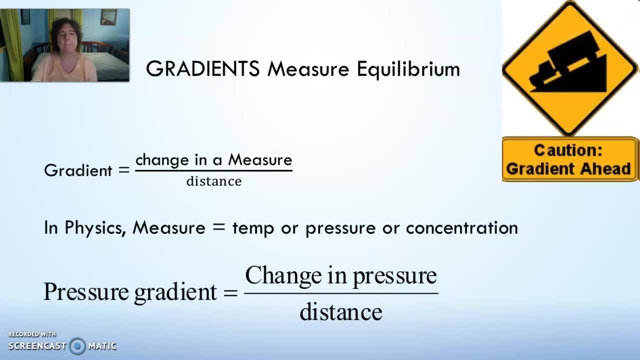 pressure to low pressure is actually a pressure force that moves that material, So let's discuss that a bit more. When we talk about equilibrium in physics, we talk about gradients, And gradient is actually the change of a measure over the distance between those two measures. 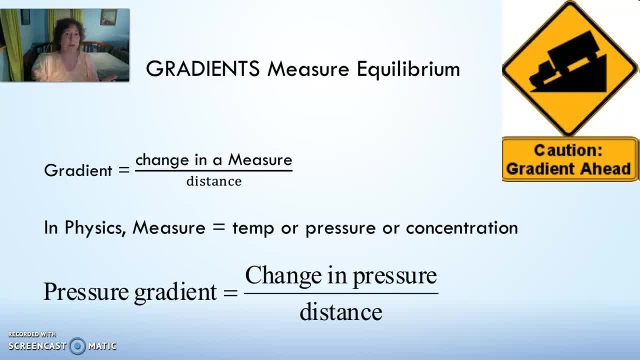 In physics that can be a temperature or pressure, like PV equals MRT, or it can be a concentration of water vapor to air. So you see that a pressure gradient that we're talking about is a pressure gradient, And when we talk about equilibrium in physics we talk about 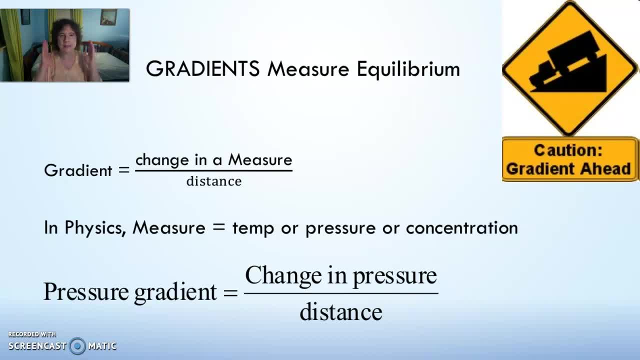 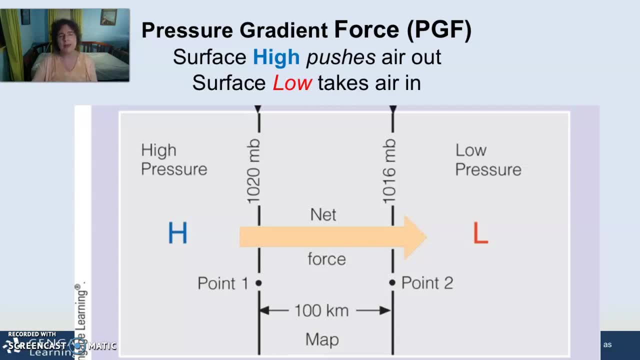 a change in pressure over distance. Let's explore that a bit more too. When we come back to this slide, we can look over a hundred kilometer distance between the pressures that are at 1,020 millibars and 1,016 millibars And the force, the net force, that moves between the high at 1020. 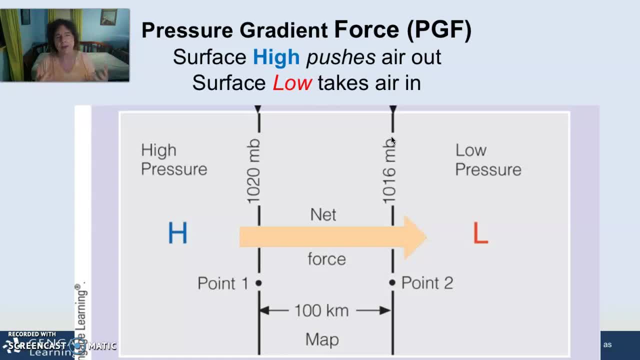 and the low at 1016, is known as the pressure gradient. So we can look over a hundred kilometer distance between the pressure gradient force. That pressure gradient force pushes out the air from the high pressure area and pushes it into the low pressure area to bring it to equilibrium. 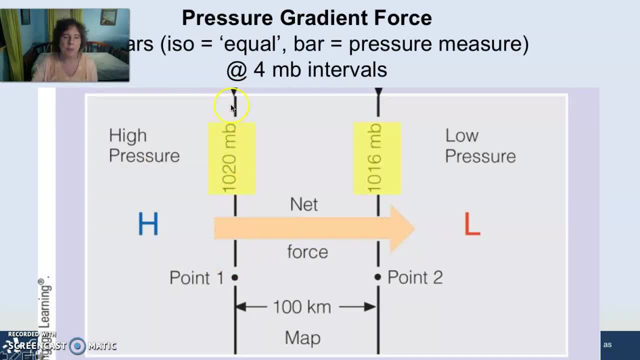 When we look at this, we can also remember that these are isobars. Iso stands for equal and bar stands for pressure, like barometer or barometric pressure, So we talk in terms of isobars. on a map that shows distance, The isobars are usually in four millibar increments. 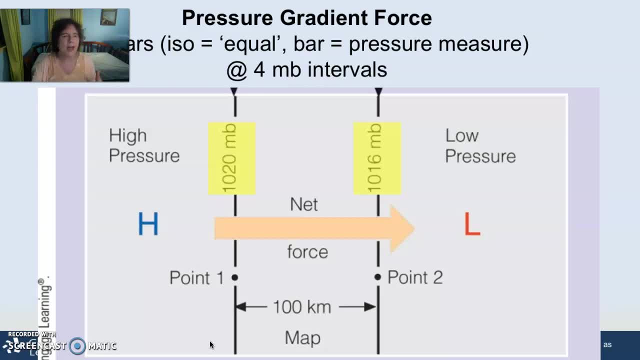 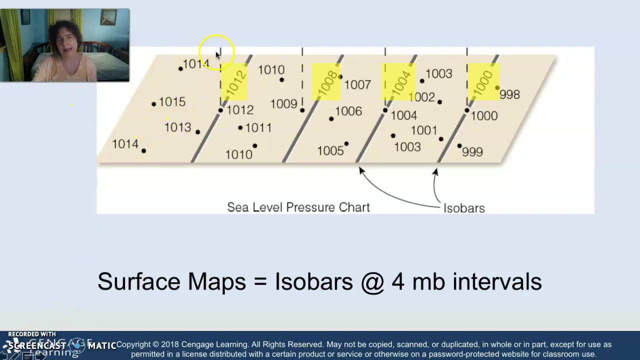 and those can range from 1020 to 1016 to 1012 to 1008 to 1004, like that, You'll see them over a wide range. For instance, you can have many measurements in between the 1016 that would be. 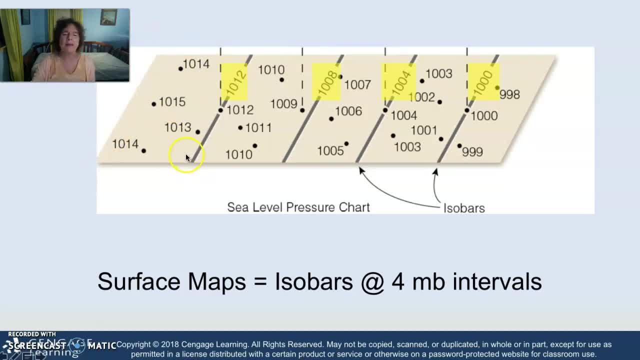 here and the 1012 and you can have many measurements in between the 1012 and the 1008 and those measurements all fit in and then you can connect the dots between the 1012 and you connect the dots between the 1008 measurements and 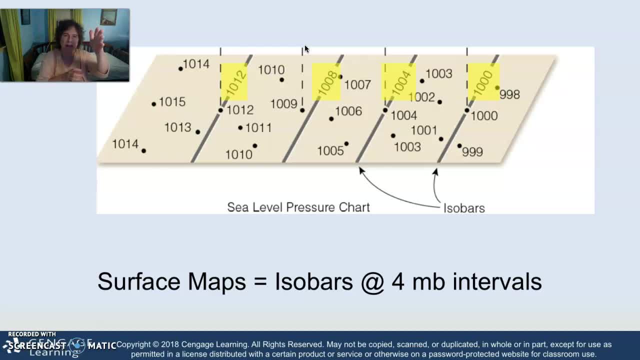 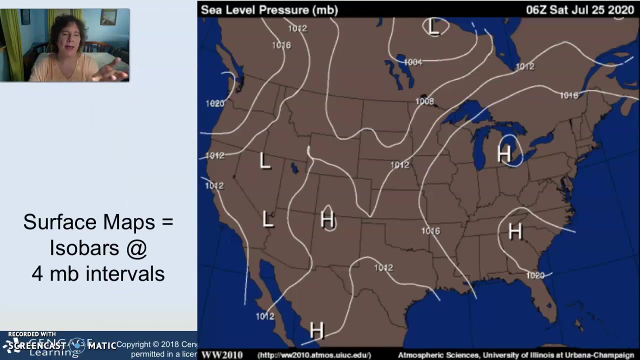 then all the rest of them fit in between there on a continuum. but these are for surface maps only and surface maps deal in ISO bars of anything from 950 millibar pressures at the surface to 1050 pressures at the surface. just play that a bit more. when we go to a surface map of the United States we might find a. 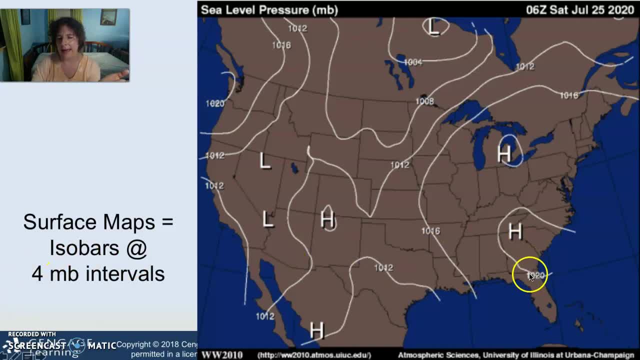 line like around South Carolina here, and that's it combining all a line that matches the map is different from how we would want it to look like in the 10-20 millibars all in this line. So I might have a measurement here. that's 10-20, a measurement. 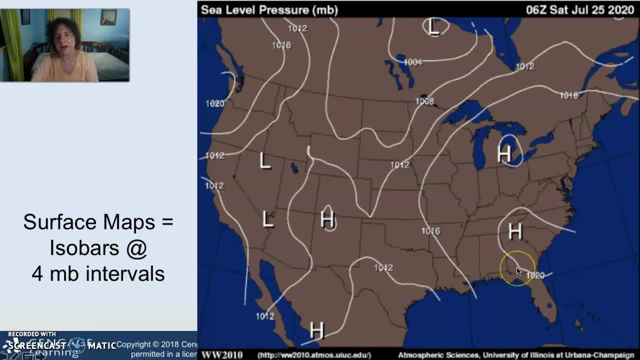 here, that's 10-20, one here and one down here, that's 10-20.. And I make a line like connect the dots. The lines are not perfect And in fact we make them so that we can fit in the other. 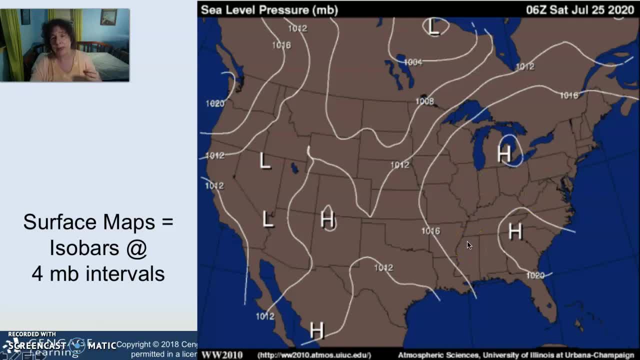 pressure points in between. So in here will be 10-19, 10-18, 10-17.. And then there will be a point here that's 10-16,, a point here that's 10-16,, maybe one here that's 10-16, here maybe one here. 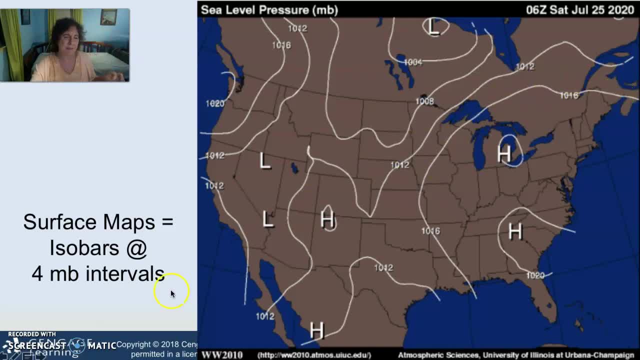 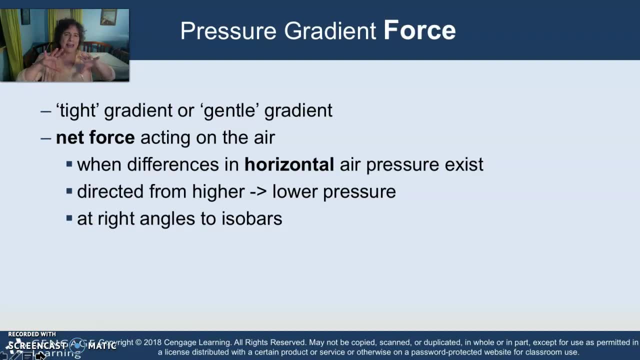 that's 10-16.. I can connect the dots for 10-16.. So that's an isobaric map And that talks about the net force that is made up of the pressure points. So I can connect the dots for 10-16.. 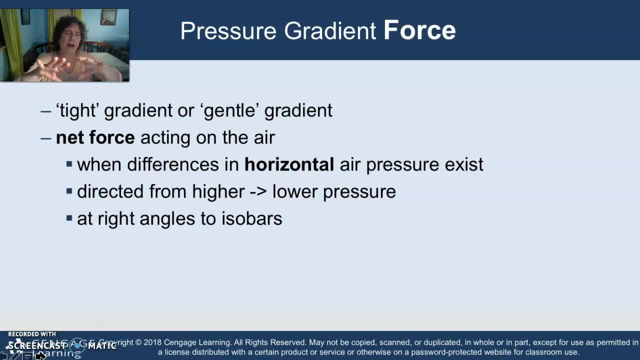 Moving between that high pressure area and the low pressure area. Now it may not look like it's talking about the net force, but what you're looking at is the difference between a gentle gradient in some areas and a tight gradient in other areas. Let's explore that a bit more. 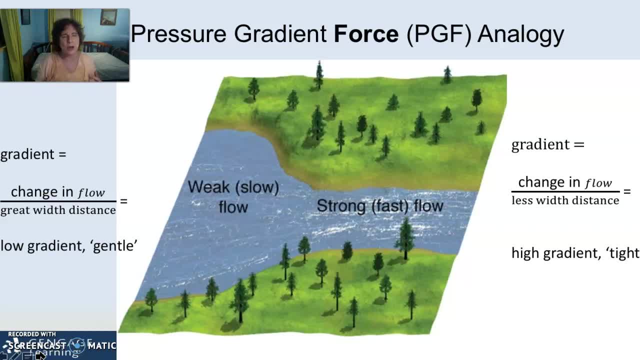 When we talk about gentle gradients, we're talking about a change in flow over a distance, because that's what a gradient is: While you have a great distance between the shores of your flow, here you'll have a large denominator. When you have a large denominator, your quotient is going to be. 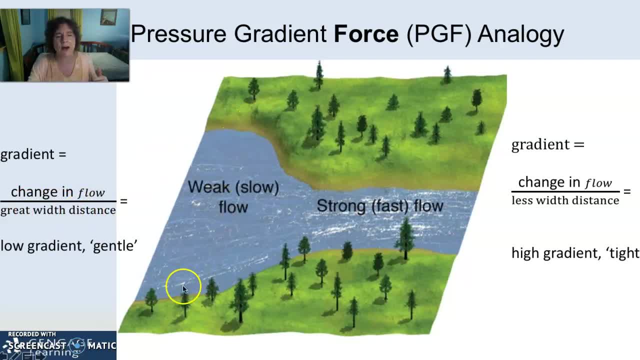 low. There's going to be a low force here to move this water through the gap. But when you come in here, where there's a very small distance between the shores, you've got a much smaller distance here, leading to a bigger quotient or a bigger gradient force. 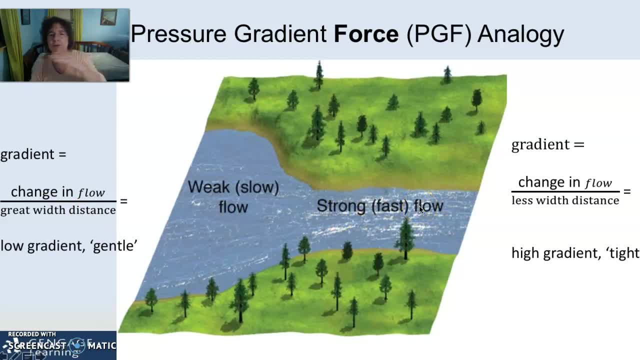 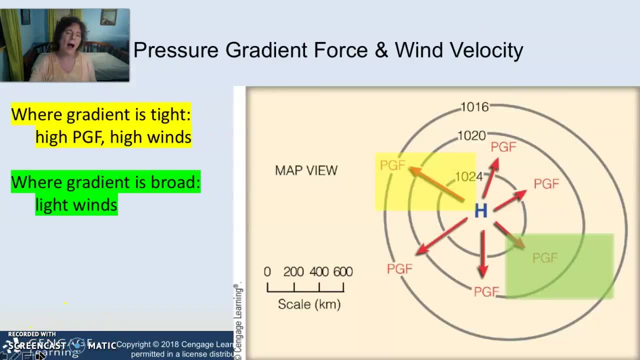 And you will notice in here that there's a faster flow in this narrow area, Very similar to what we're looking at when we look at the maps that are isobaric maps. When we have tight gradients in here, just a bit of distance between the shores, you'll have a much smaller gradient force. 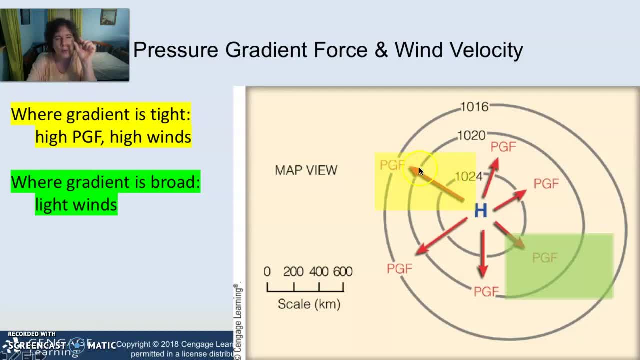 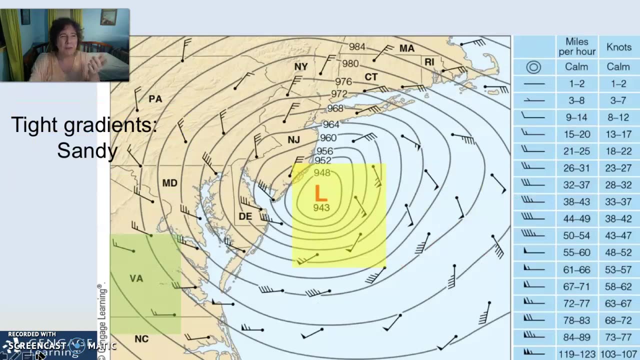 When we look at the isobaric maps, when we have tight gradients in here, just a bit of distance between the shores lines, in between the isobaric lines, we have stronger winds, and when we have a broad area between the isobaric lines, we have gentler winds. in here you might. 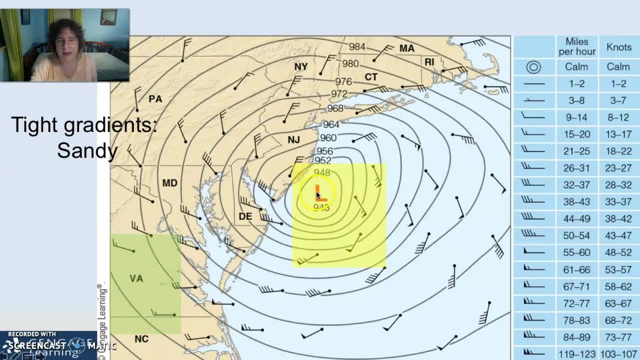 remember sandy, and what I wanted to point out here is where the gradients are very tight in through here- not a lot of distance between the lines- the winds are much higher. you can even check them out over here. the winds are higher speed where the isobaric lines are very tight and where the isobaric lines are broad. 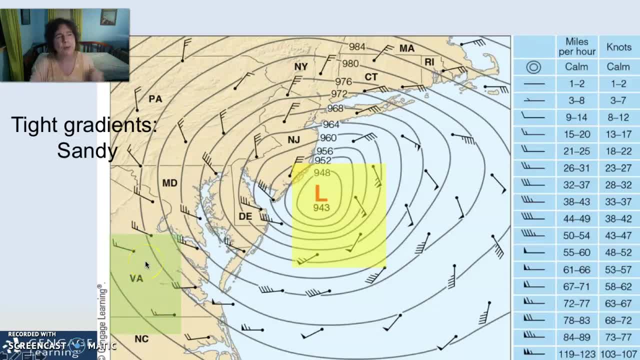 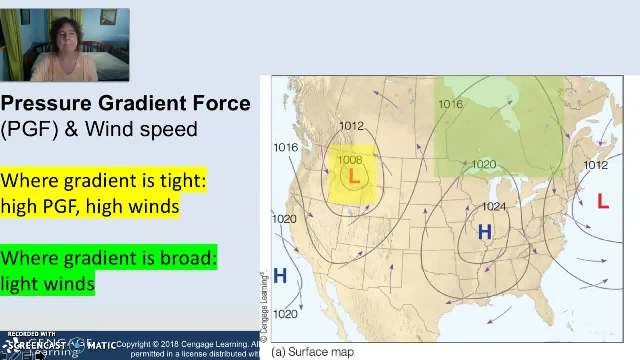 with a lot of distance between the lines, those winds are going to be quite a bit lighter again. this is a surface map and I wanted to point it out to you nationally as well, that where you find the highest winds are the ones that are higher, and where you find tighter on tighter gradients, you will find speeds. 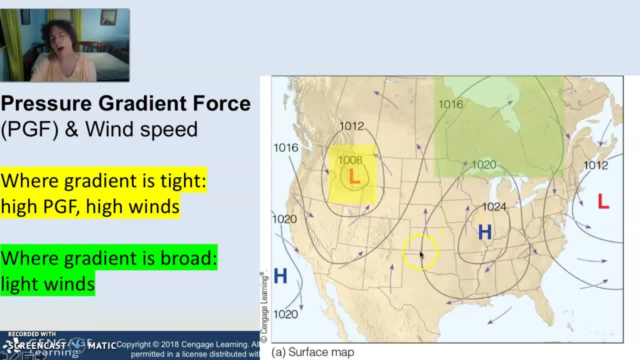 that are higher and where you find broader gradients. especially up in here, you're going to find winds that are lighter. now this map does not tell you about the speeds of the winds. this map tells you about the direction of the winds, but I wanted to give you an overall view of tight gradients versus. 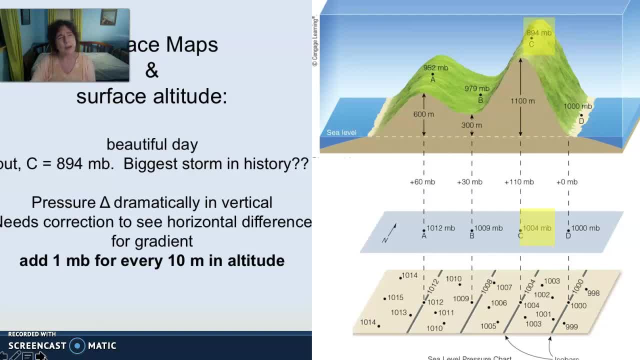 gentle gradients. there's one last thing they need to talk about with pressure and that is surface altitude and how it affects surface pressures and surface maps. now you see here, this is a beautiful day and you might think there's not a cloud in the sky. it's a beautiful day that would probably be at a pressure. 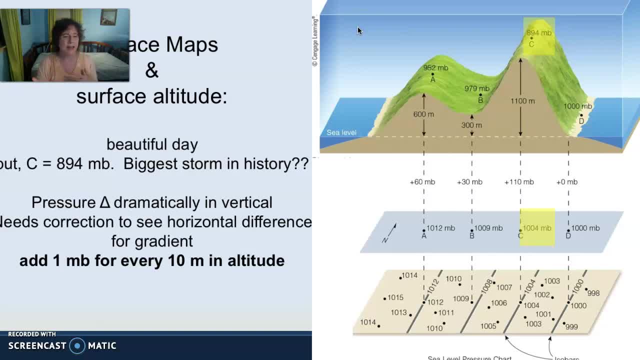 of about 10, 10 to 10, 20 or so, and but you can see here on this map that the this surface up here at sea, you get this really low pressure of 894. that low pressure of 894 would be the worst hurricane of the century, but it's not the surface. on a beautiful day and what you're. 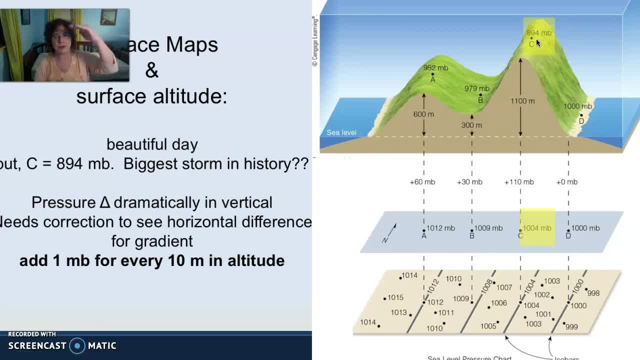 seeing is that there's a very dramatic change in pressure over altitude. remember our graphs that looked at temperature and altitude. that pressure, that temperature change was very steep as altitude increased. so in doing that we have to correct for um changes in a vertical pressure and we have to do that in order to see the differences on an even playing field. 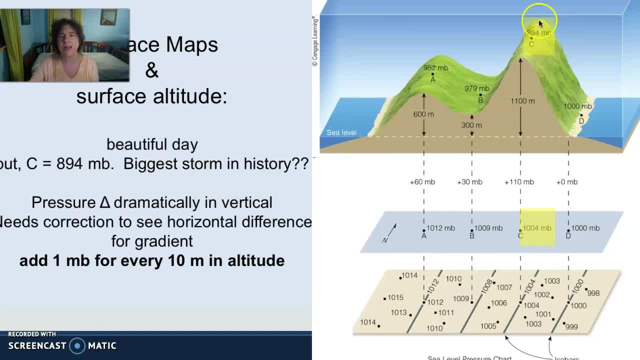 on a surface map. the way we change and correct for those pressures is to look at the altitude. this altitude is at 1100 meters and we say to ourselves, okay, for every one, um, for every 10 millibars of altitude, i'm going to add one millibar of pressure. so what you? 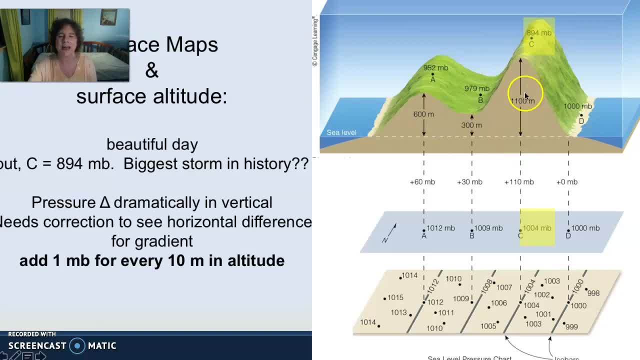 do. when you look at the altitude here, you just take off 10 and you say, okay, i will add in 110 millibars of pressure for 1100 um meters of altitude. so i just divide by 10 and i put and add on that. 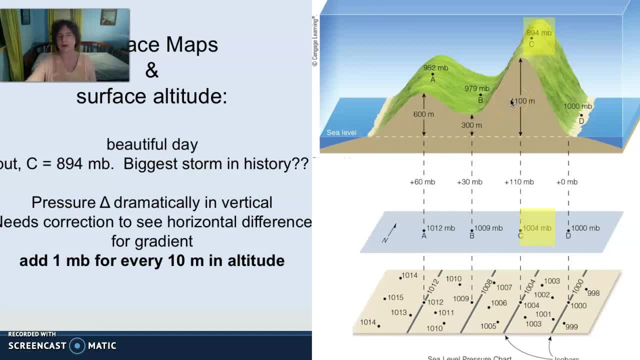 110 millibars of pressure. so when i add 110 millibars of pressure to 894 millibars, i'm actually getting 1004 millibars, which is a really fair weather pressure and i can compare it to other pressures right at the surface at a thousand millibars, and i can compare it to other pressures.